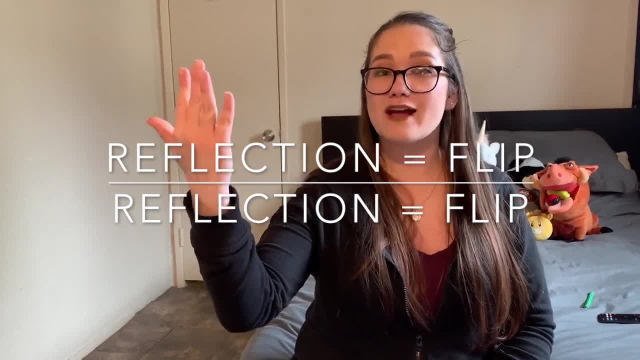 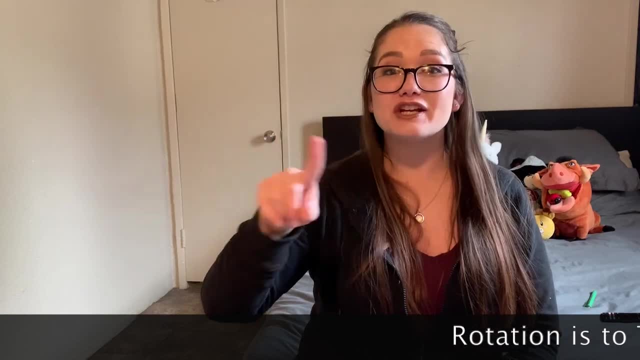 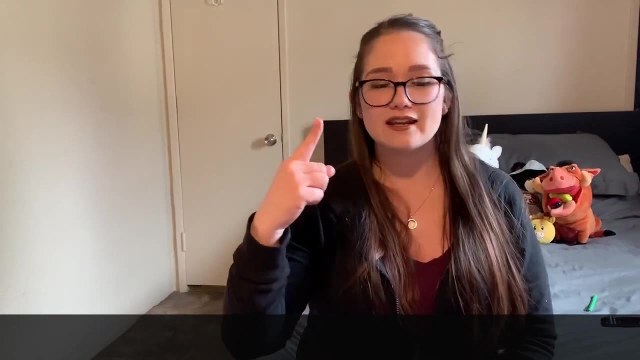 you got to flip. Okay, The word is flip, Reflection is to flip the figure. Okay. You have to do the head, Okay, And then rotation, you have to turn. Rotation is to turn, Rotation is to turn, Rotation is to turn around at a point. And, yes, the head is a must. So let's get into the actual 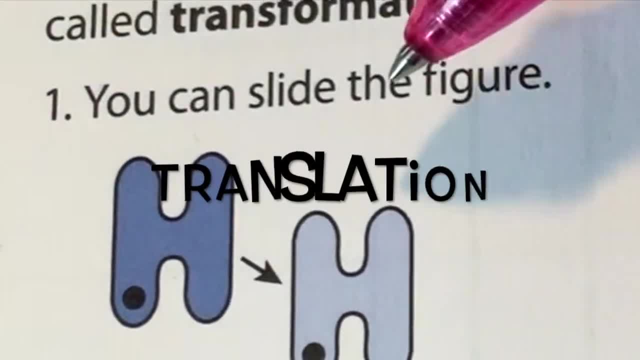 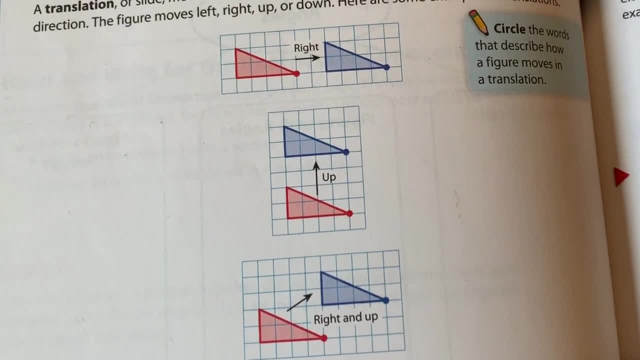 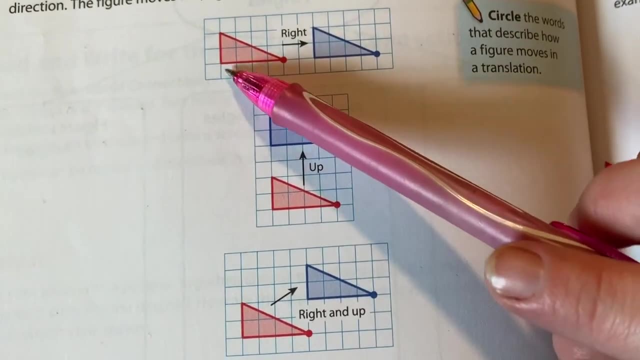 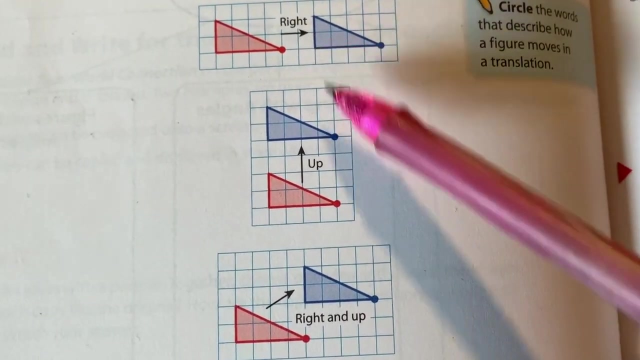 math part of it. So this one here is a translation. And again, translation is a slide. A translation or slide. It moves every point of a figure, So the whole figure moves. Point A, B and C move, And point A, B and C look the same. Okay, It's the same distance in the same direction. Okay, If the 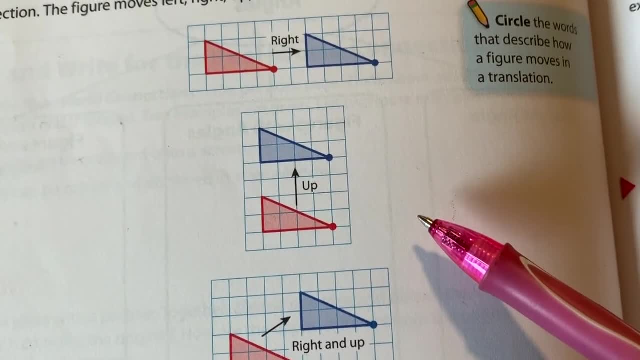 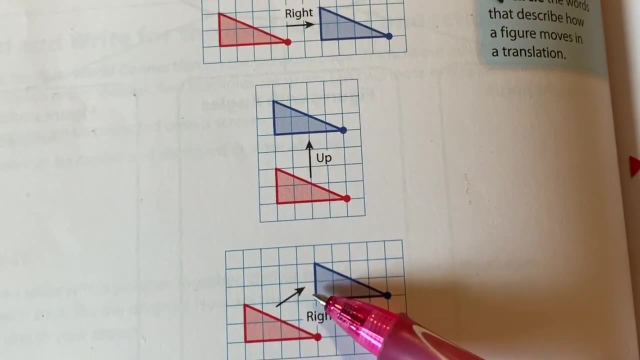 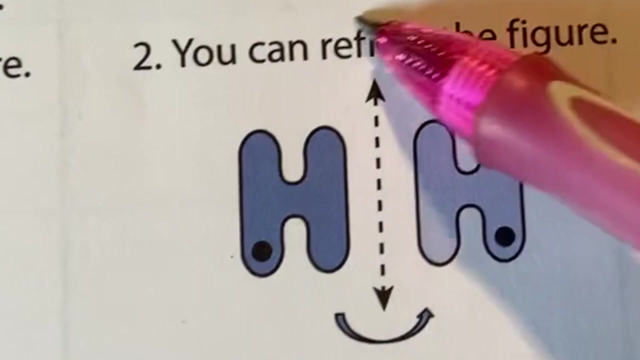 figure moves left, right, up or down. And then here are the examples: If it moves right, if it moves up, if it moves up and to the right. Okay, The next one: here is a reflection And you're reflecting. The dots here means that this side of this figure is a reflection And you're reflecting. 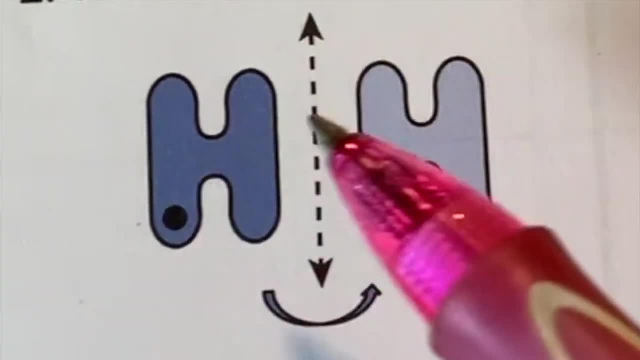 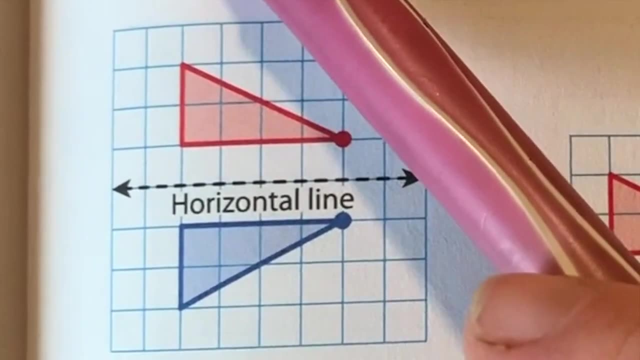 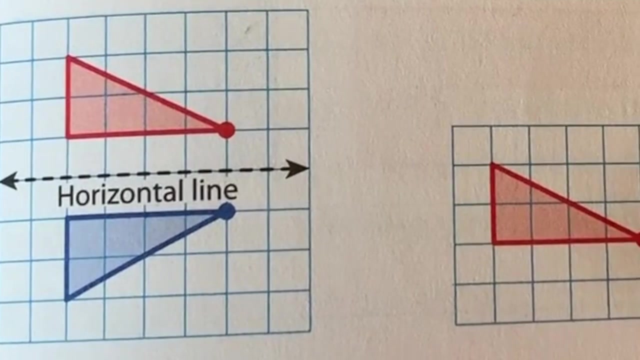 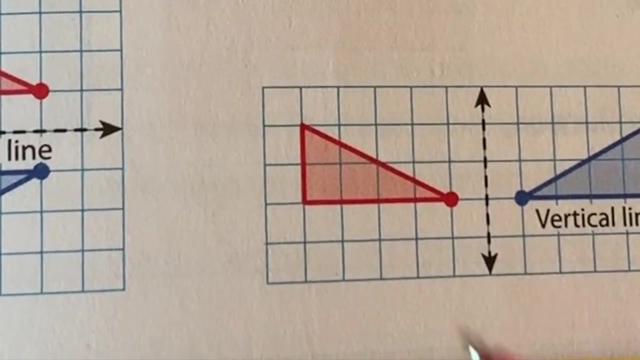 this side of the H, So it literally flipped over. Remember, a reflection is a flip. Reflection was a flip. Okay, Just like that mirror. A reflection it's a flip. Okay, It's across an imaginary line. Okay, It can be a horizontal line, a vertical line or a slanted line. The line is called the. 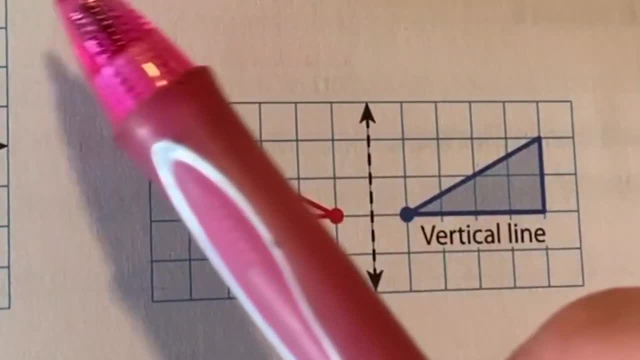 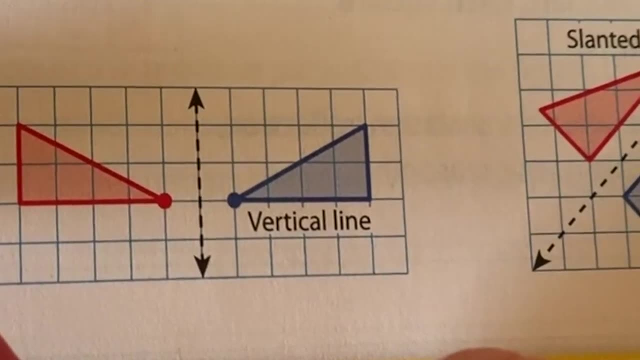 line of reflection. Okay, So the original figure and its image would match exactly. Okay, So it's not going to be smaller, It's not going to be bigger. The image is going to be exactly the same. It's just going to flip. 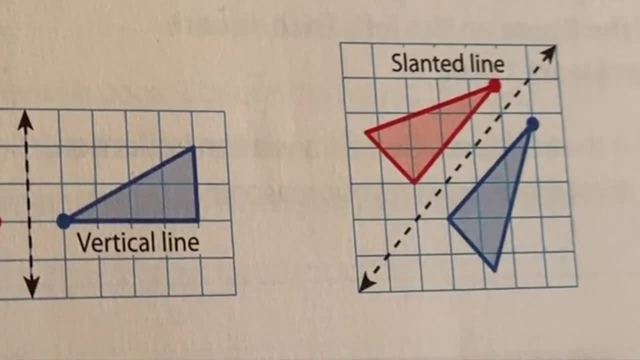 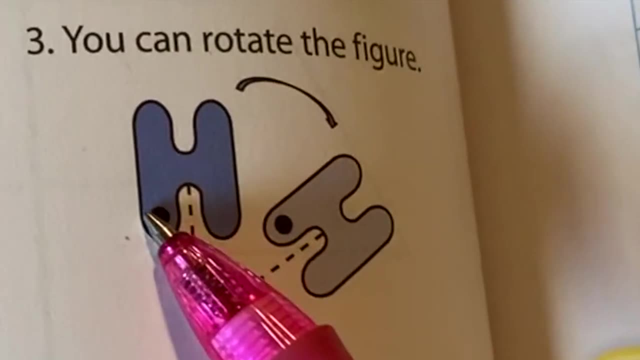 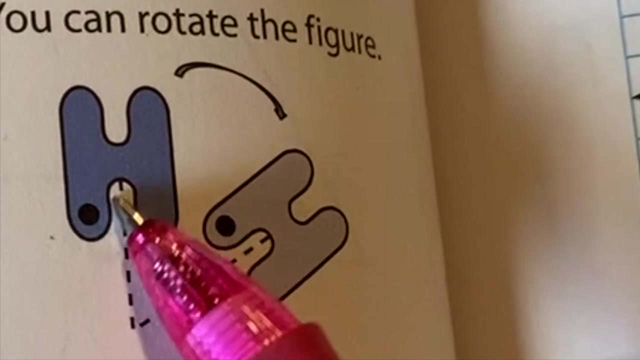 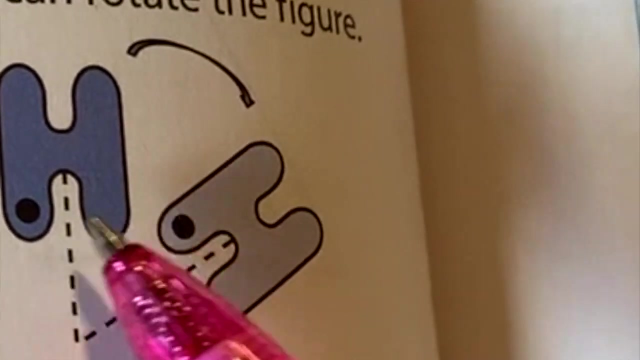 across an imaginary line or a line of reflection. A rotation is a turn. So, remember, we did that little turn with our heads. It starts at a point and it turns about a different point. Okay, It rotates this way, And this part of the H is now this part of the H here. Okay, So it did that.